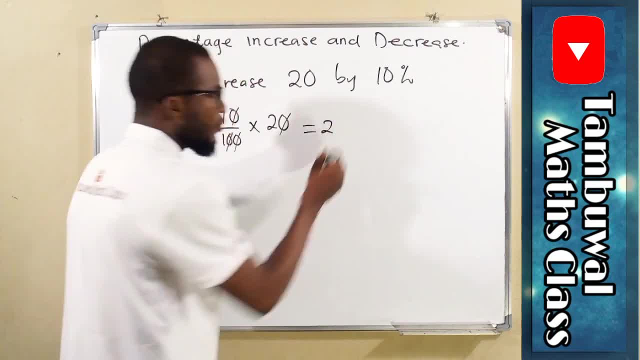 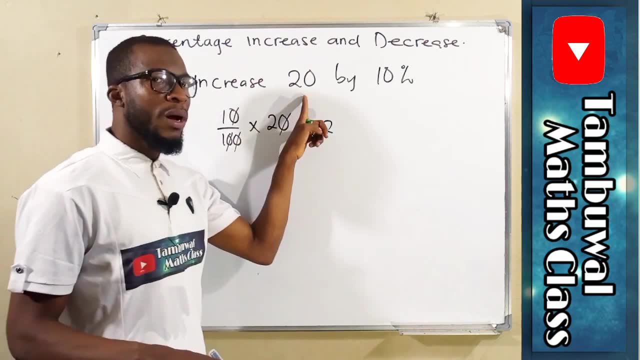 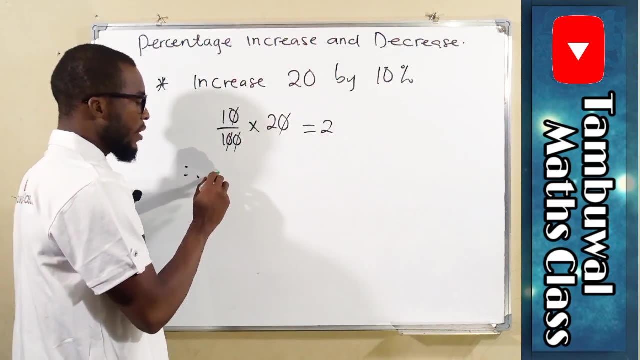 What we have left is just: 1 times 2 equals 2.. This means that 10% of 20 is true, But the question says we should increase the number by 10%. We have already obtained the 10%. Therefore, we have 20 plus 2, which is equal to 22.. 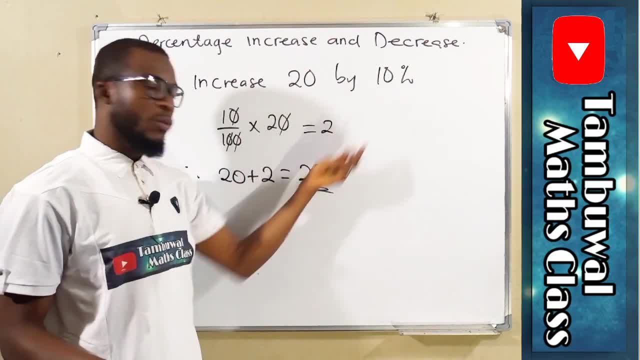 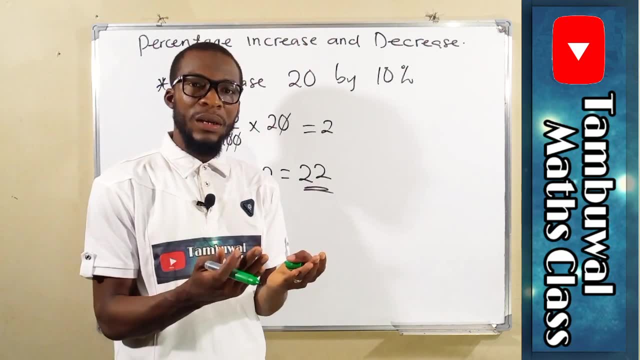 So if we increase 20 by 10%, we are going to obtain 22.. So if we increase 20 by 10%, we are going to obtain 22.. Another approach: remember I told you, every number in its original form is 100%. 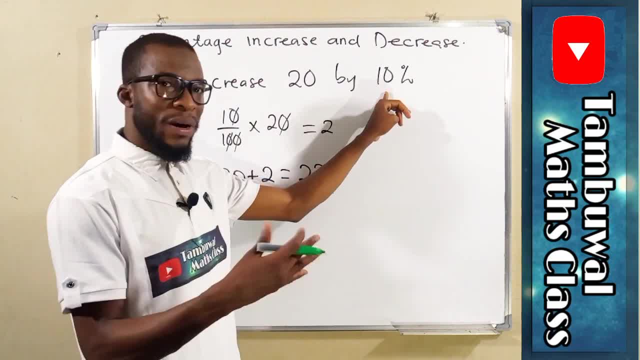 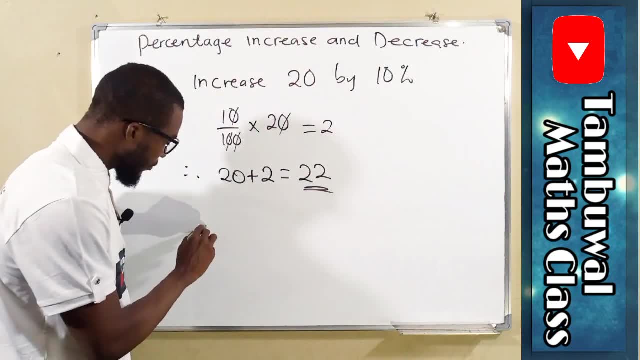 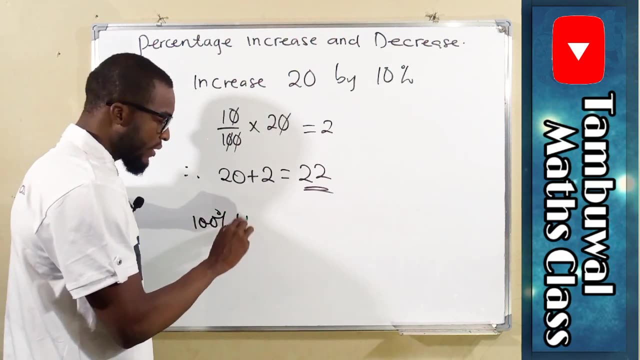 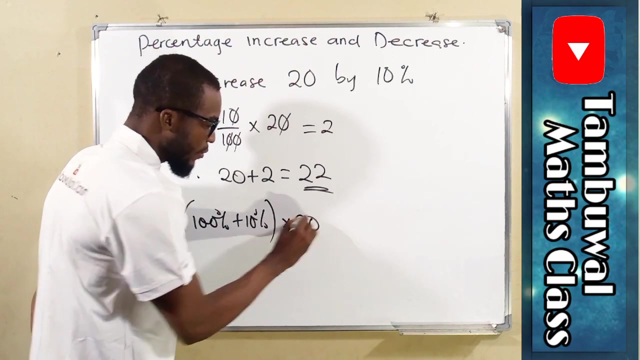 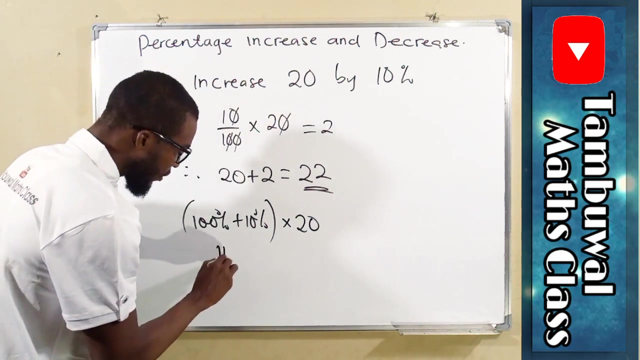 So to increase that number by any percent, all you need to do is to add that required percent to the 100.. So we have 100% plus 10% of what we have here. What we have here is 20.. And you can see this is 110%, which can be written in rational form as 110 over 100 multiplied by 20.. 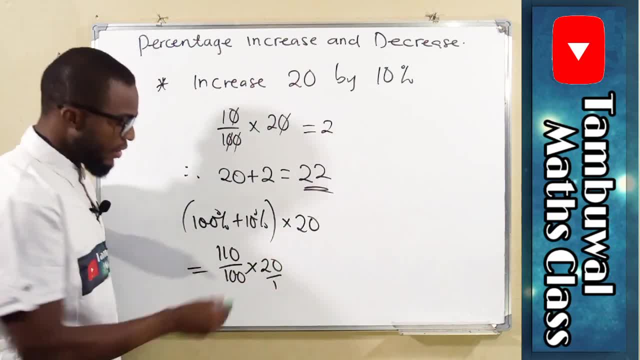 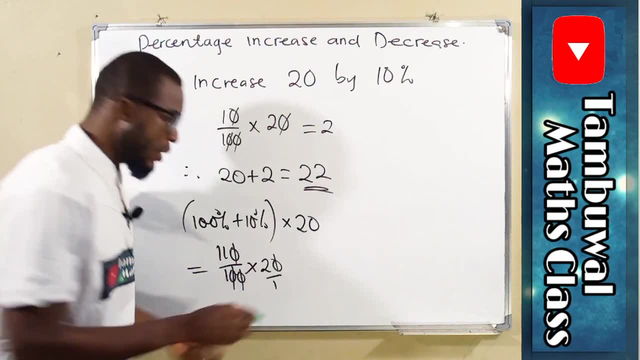 You can rationalize it if you like: 0 here, 1. 0 here, 1. 0 here, 0 here. All we have left is 11 times 2, which is the same thing as 22.. So these are the two approaches. 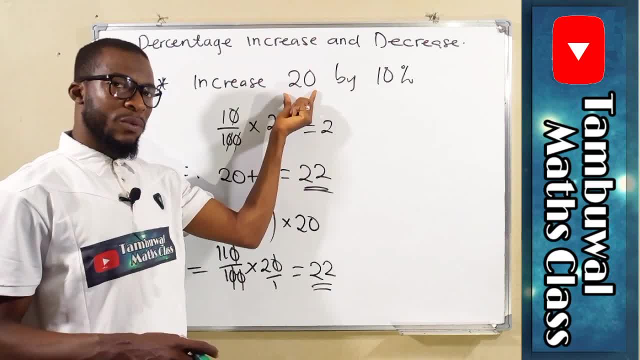 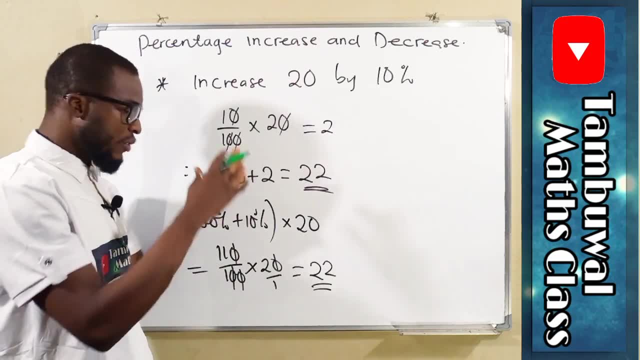 It's: either you find the 10% of that number. whatever you obtain, you add it to the original number, Or you increase the percentage because its original form is in 100%. We want to increase it to 110 because we are adding 10.. 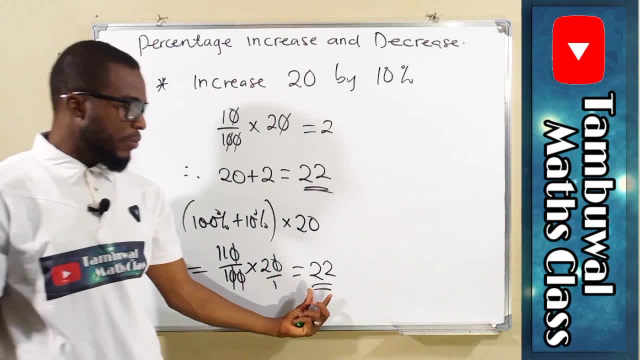 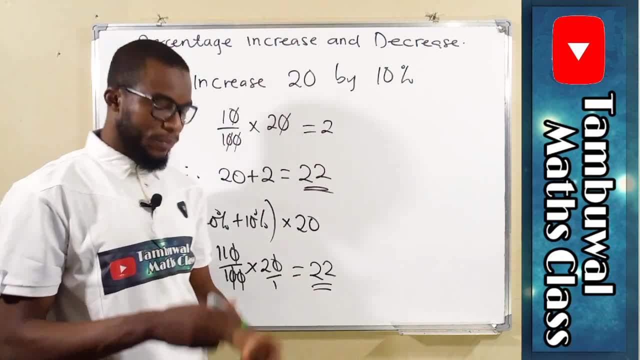 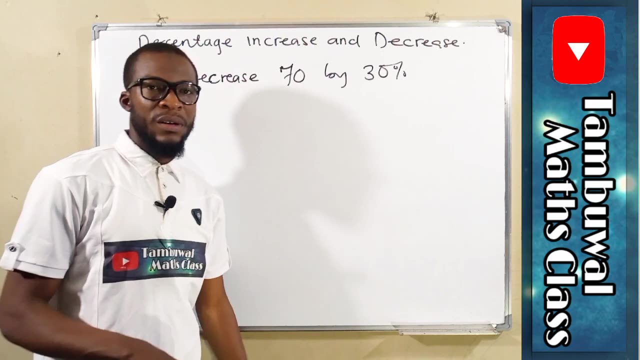 So we have 110% of that number, which is the same thing as 22.. So now let us see how we can find the percentage decrease of a number. So this question says we should decrease 70, which is a number, by 30%.